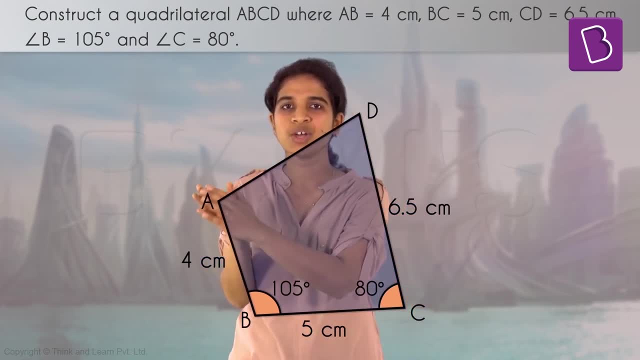 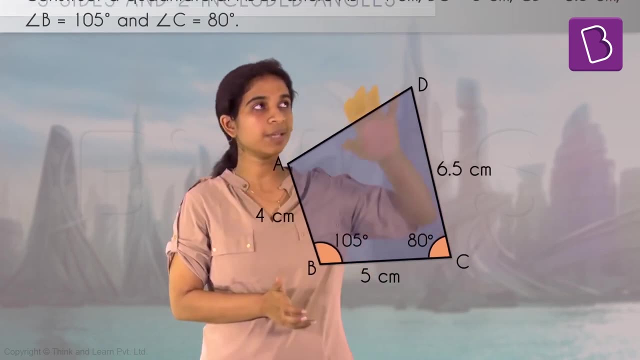 Same concept. again, Go back to what you know about triangles. When you use some sides and some angles in a triangle, use the exact same thing and we'll draw this quadrilateral. So let's keep this figure here for our reference. That's always important Before you start constructing a. 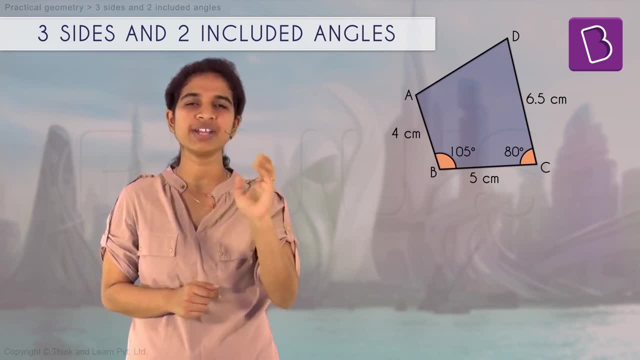 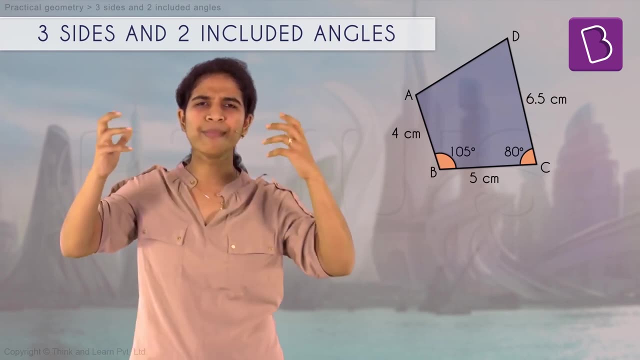 figure. just always draw a rough sketch and mark out the information that is given to you and use it as a reference when you're doing the actual constructions. Makes it much easier, Rather than trying to imagine the figure from a sentence that is written on a paper in front of you. 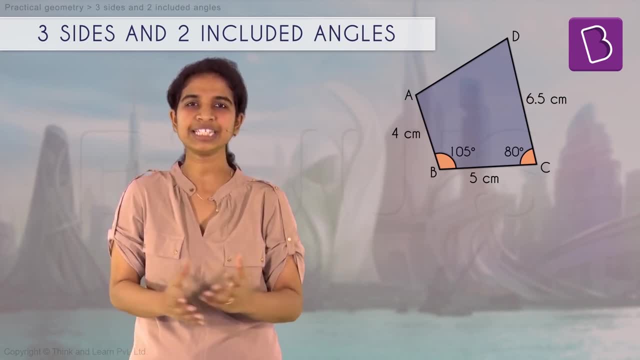 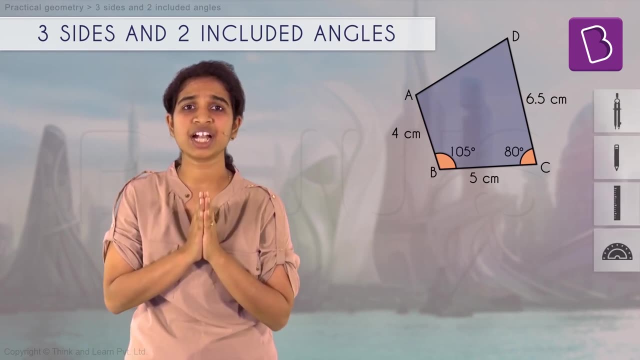 just draw a rough figure Makes it much simpler. It is practical geometry at the end of the day, right? So let's get practical. Let's not have sentences, Let's have just diagrams. Okay, so let's get started. Where do we start? There are three sides. We know that. we always 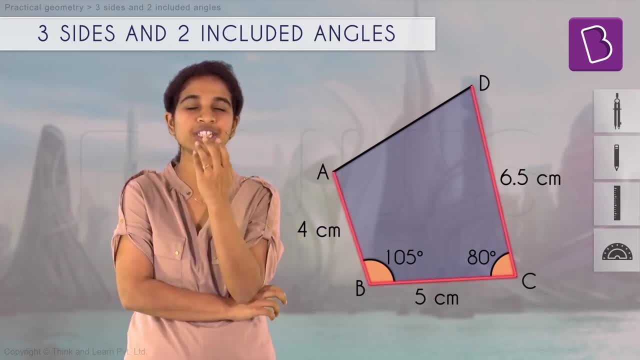 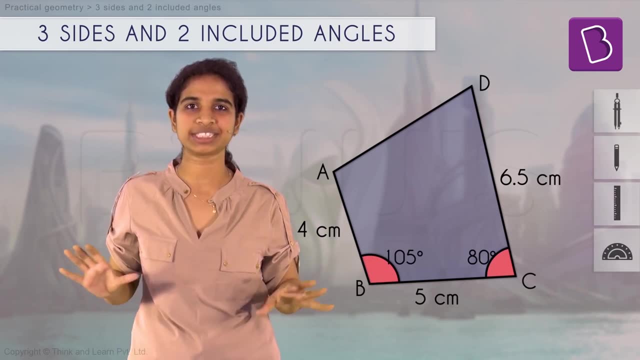 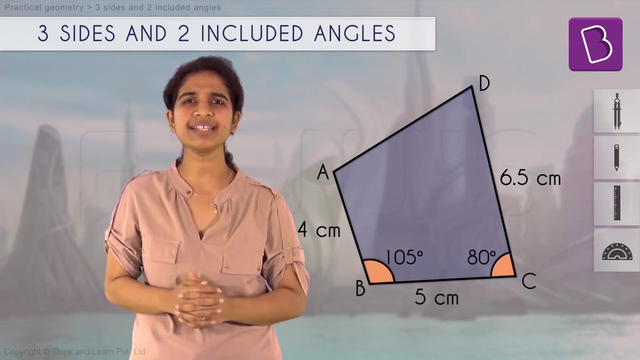 start with a side. Now there are three sides given. What side do we start with? What side do we start with? What's the rule? We start with a side where we know the angles on both sides correct. Only then we can proceed. So let's start with a side where we know the angles on both sides Makes it. 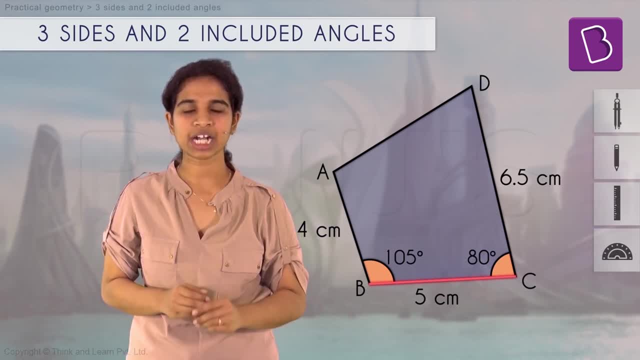 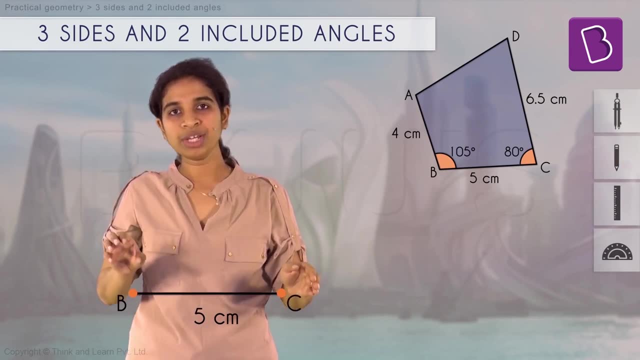 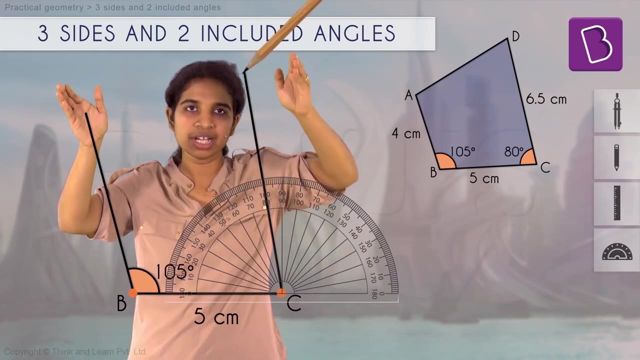 easier that way. So we'll start with BC. Let's start with BC. So mark point B here, Draw a line. you have point C here. Now we know the angles on both these sides, right, We know angle B, we know angle C. So at B, draw 105 degree angle, At C, draw 80 degree angle. So you have both of. 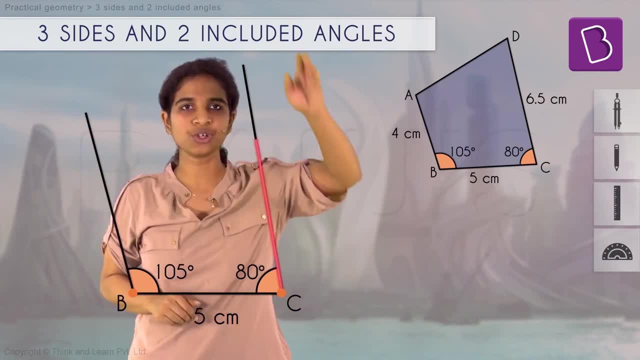 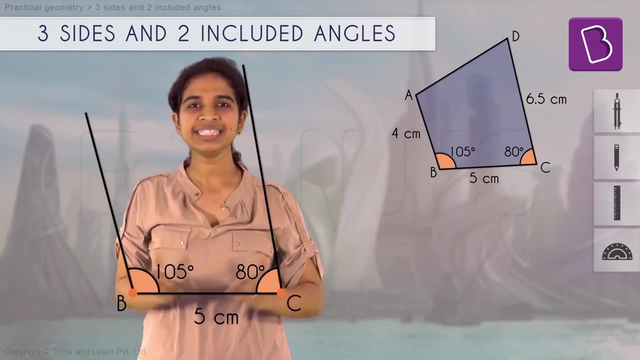 these angles. A is going to lie somewhere on this line, D is going to lie somewhere on this line. Can we find out exactly where A lies and exactly where D lies? Yes, very, very simple, right, Because we know the lengths of both of these line segments. So this is actually easy, much easier. 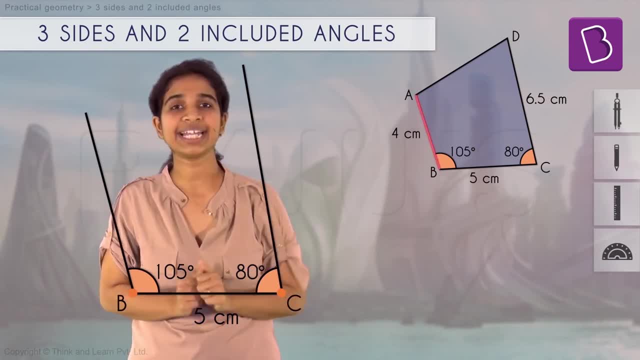 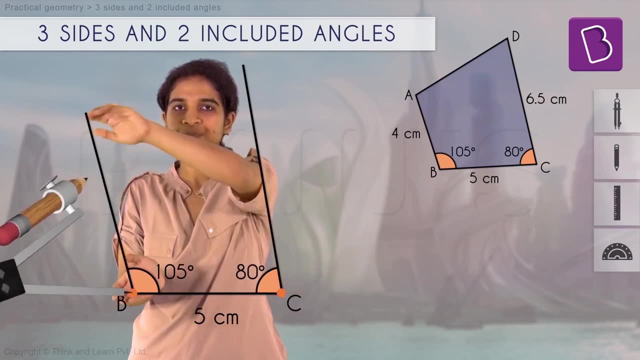 than the previous one, because we know the exact lengths. It's given to us that AB is 4 cm. So take your compass, measure 4 cm. keep one leg of the compass at B, draw an arc Wherever it cuts this. 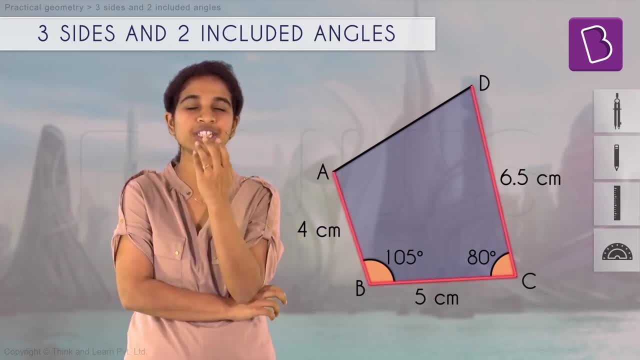 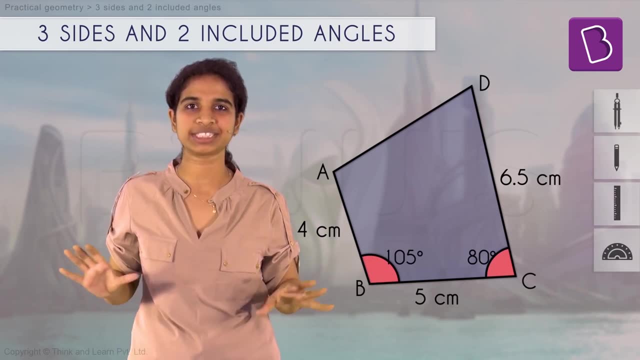 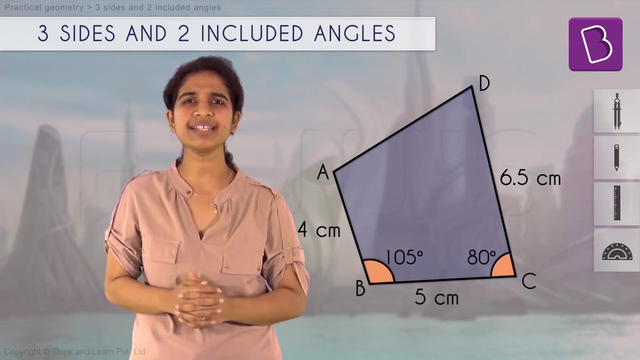 start with a side. Now there are three sides given. What side do we start with? What side do we start with? What's the rule? We start with a side where we know the angles on both sides correct. Only then we can proceed. So let's start with a side where we know the angles on both sides Makes it. 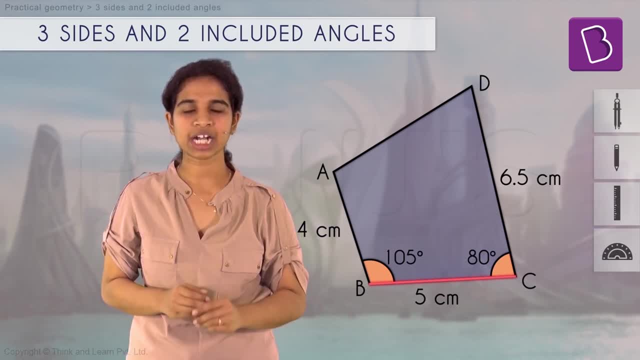 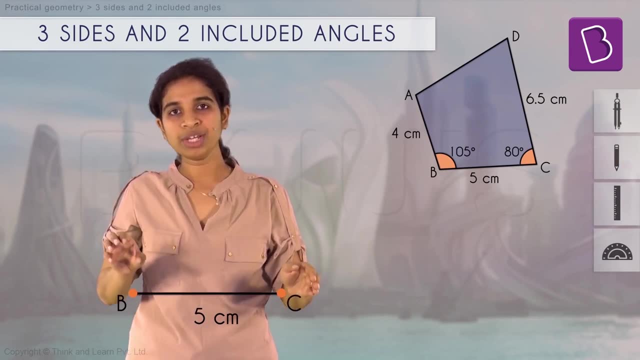 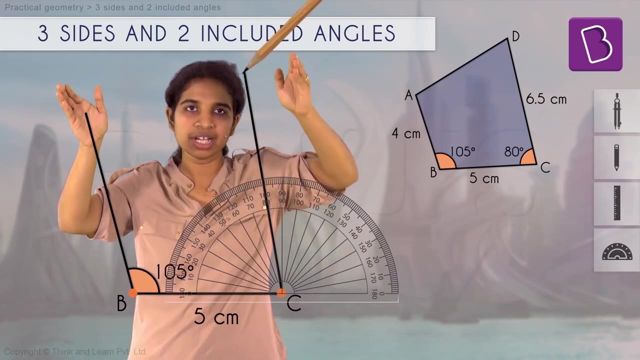 easier that way. So we'll start with BC. Let's start with BC. So mark point B here, Draw a line. you have point C here. Now we know the angles on both these sides, right, We know angle B, we know angle C. So at B, draw 105 degree angle, At C, draw 80 degree angle. So you have both of. 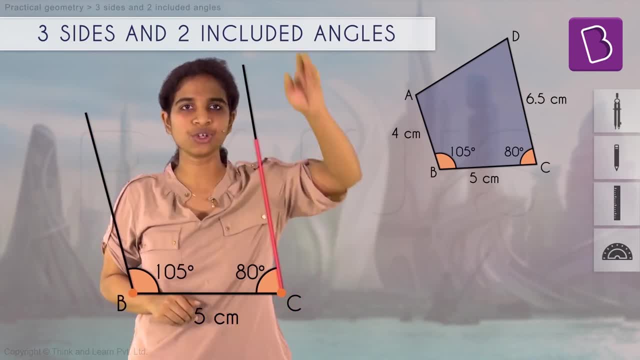 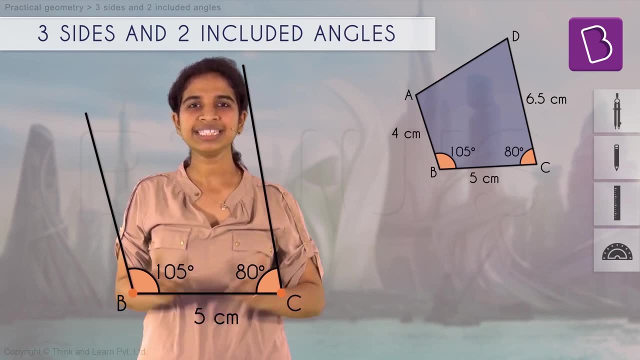 these angles. A is going to lie somewhere on this line, D is going to lie somewhere on this line. Can we find out exactly where A lies and exactly where D lies? Yes, very, very simple, right, Because we know the lengths of both of these line segments. So this is actually easy, much easier. 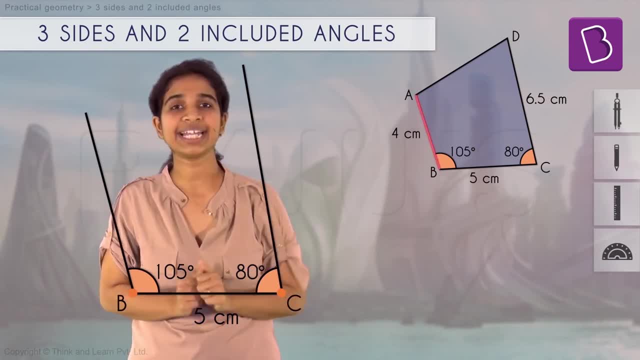 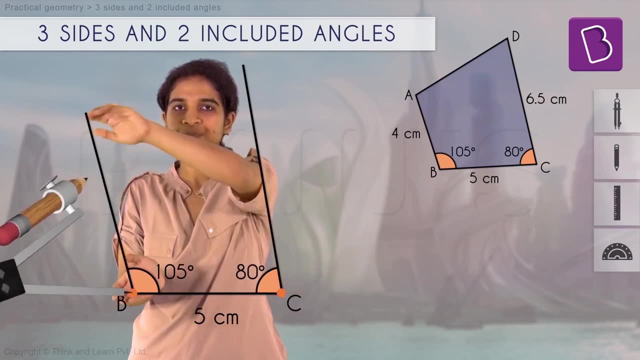 than the previous one, because we know the exact lengths. It's given to us that AB is 4 cm. So take your compass, measure 4 cm. keep one leg of the compass at B, draw an arc Wherever it cuts this. 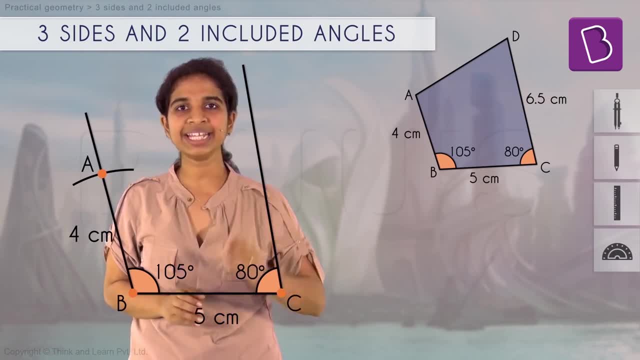 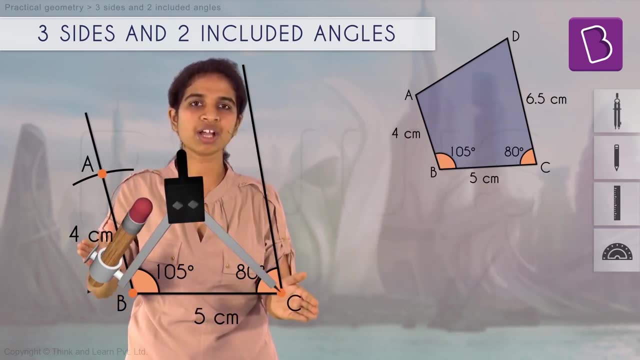 line, you get your point A. Similarly for drawing CD, how much are you going to measure in your compass? Measure a length of 6.5 cm, keep one leg of the compass at C and draw an arc Where it. 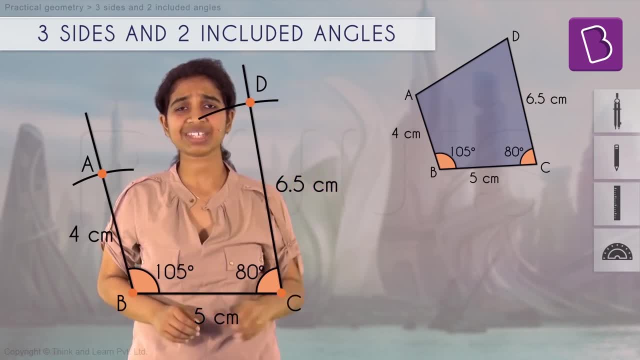 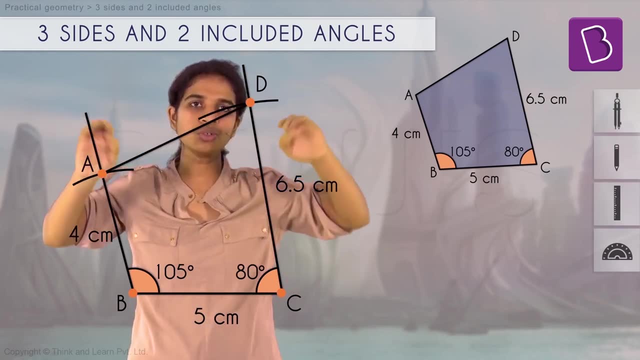 cuts. the angle that you drew is nothing but point D. It's nothing but point D. So now you have BC you already had. Now you have A and you have D. So join these two, Join AD and you have your quadrilateral ABCD, where you knew three sides. 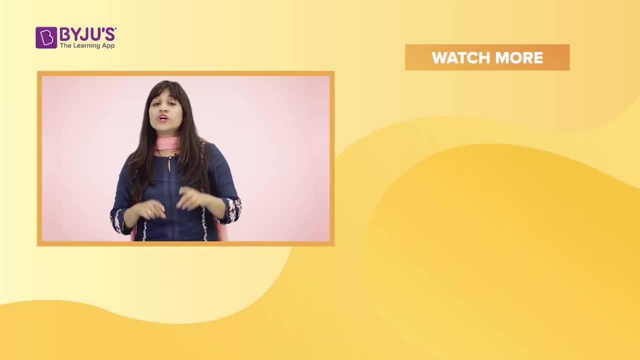 and two included angles. If you like this video and want to watch many, many more amazing videos like these, like and subscribe to our channel now. 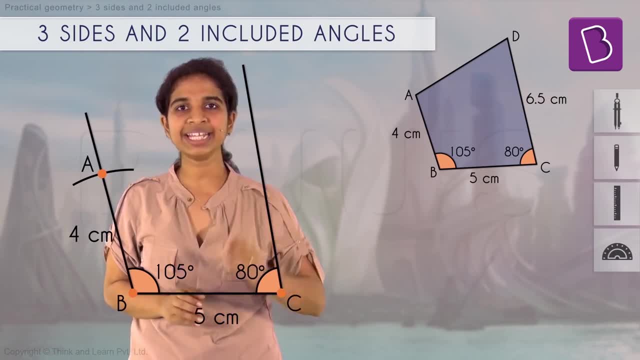 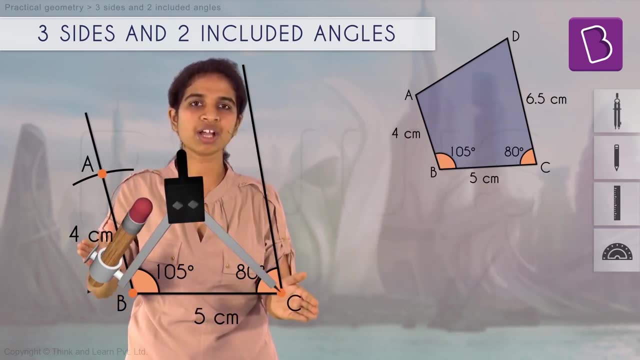 line, you get your point A. Similarly for drawing CD, how much are you going to measure in your compass? Measure a length of 6.5 cm, keep one leg of the compass at C and draw an arc Where it.